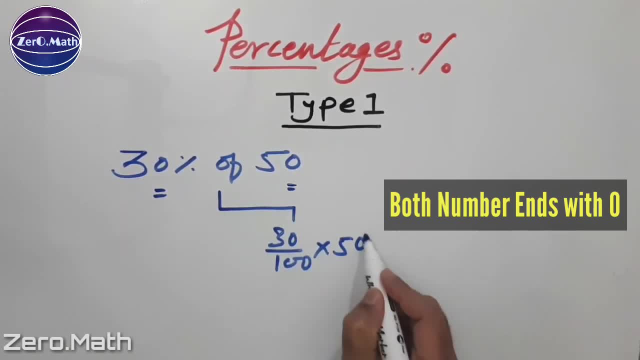 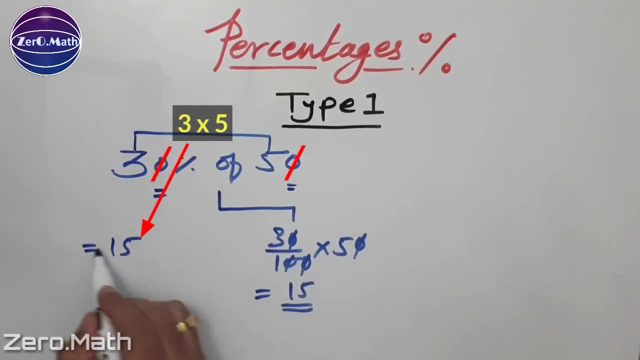 Divide it by 100 into 50.. So let's cancel out zero. 5 into 3, 15 is my answer. However, if you want to improve the speed, what you can do- the moment you will see both numbers are ending with zero- simply multiply these two numbers. So 5 into 3, 15 is my answer, which you can note down directly. So if the problem is 80% of 110, no need to do any calculation. just 8 into 11, 88. 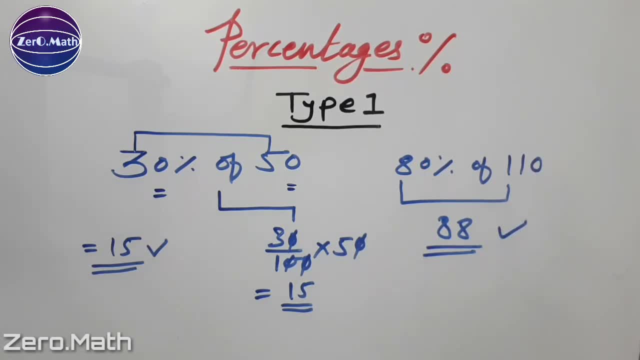 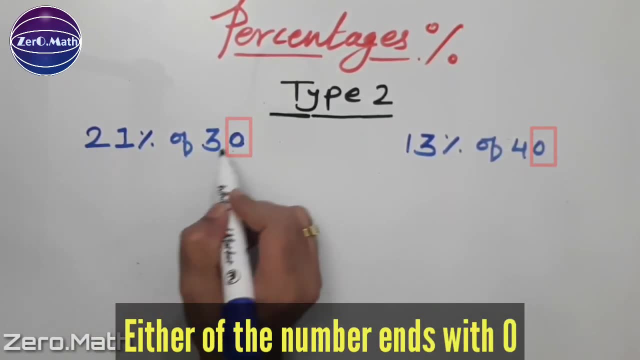 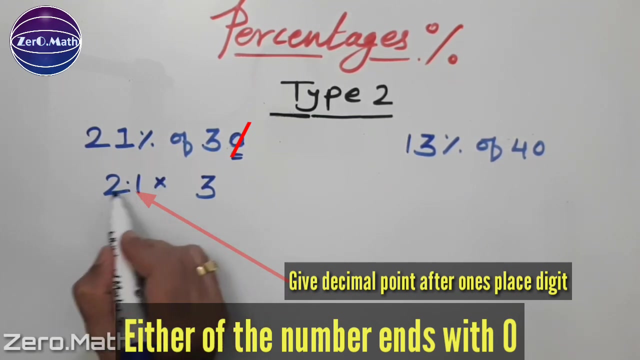 Which is my answer. Let's solve the problem of type two. So in type two, either of my number ends with zero. So 21% of 30 is 30- ends with zero. So what I'm going to do, I am going to remove zero from this 30 and I will note down this three and note down this 21 as it is, and I'll give the decimal point here after one day, So it will become 2.1.. So let's multiply 2.1 into three, which is equal to 21, into 363.. Here the decimal point is 2.1.. So let's multiply 2.1 into 3,, which is equal to 21, into 363.. So let's multiply 2.1 into 3,, which is equal to 21, into 363.. 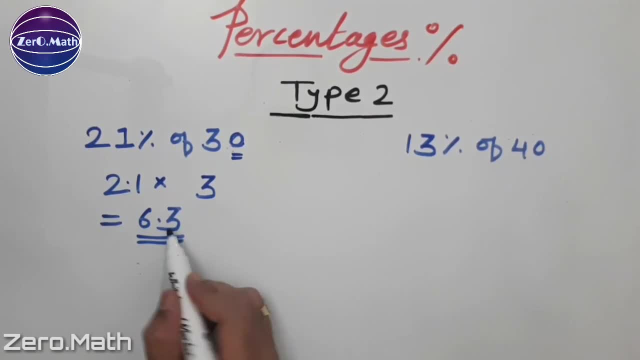 Here the decimal point after one digit, which is equal to 6.3,, which is our answer. So if one number ends with zero, you can perform direct multiplication to get your answer without performing any additional calculation. Let's calculate 13% of 40. So note down this 13 and give decimal point here after one digit into remove zero from 40 and take down this 4.. So it will become 1.3 into 4,, which is equal to 5.2,, which is our answer. 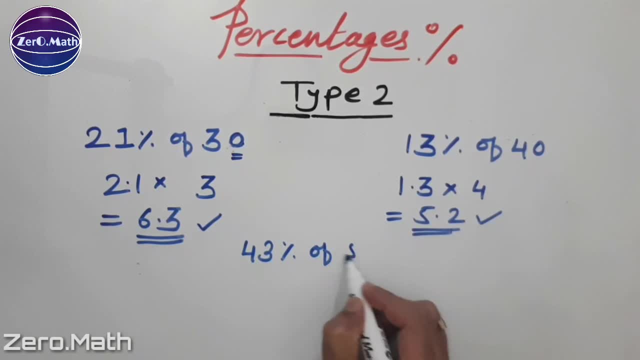 Let's calculate 43% of 40. So note down this 43, give decimal point here, so it will become 4.3 into. note down this 5 from 50, remove zero, So 44.3 into 5 is 21.5.. How to do this in mind? So let's first multiply 43 into 5. in mind How you can do this. So place value of this: 4 is 40. So 40 into 5 is 200, plus place value of this 3 is 3.. 3 into 5 is 15.. So 200 plus 5 is 215.. 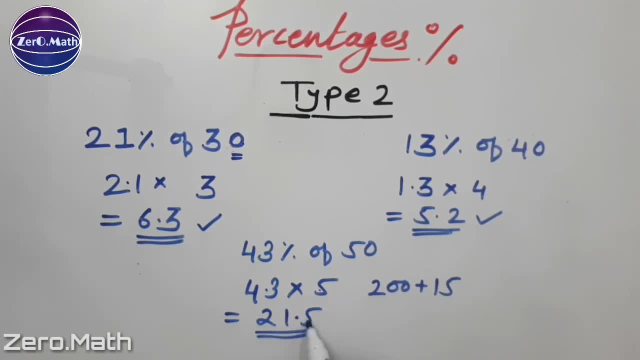 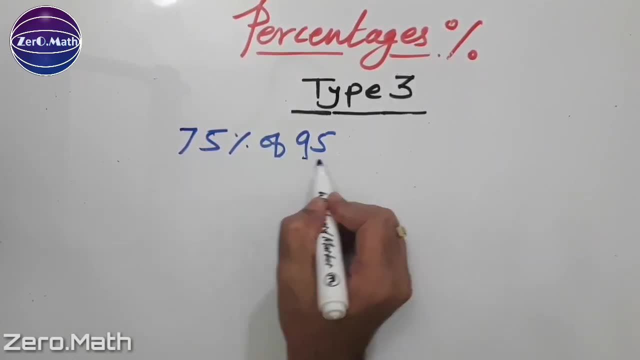 Here the decimal point after one digit, so it will become 21.5,, which is our answer. Let's solve the problem of type 3.. So in this type none of my number ends with zero. So 75% of 95, neither 75 nor 95 ends with zero. So we'll solve this using the splitting method. We'll split this 75 as 70 plus 5% of 95.. 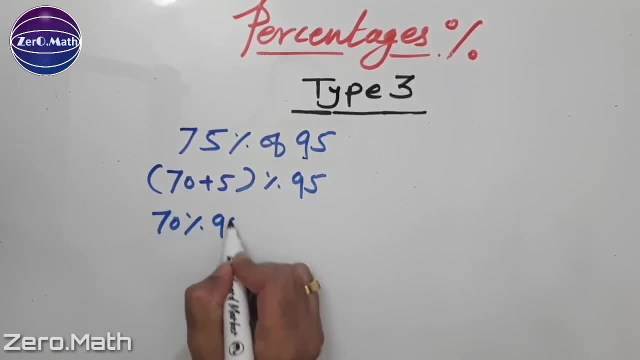 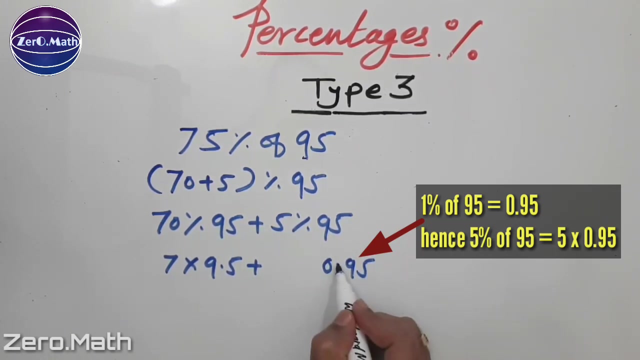 We can further simplify this as 70% of 95 plus 5% of 95. So 75, 70% of 95 is nothing but our type 2.. I can represent, I can write down the answer for this as 7 into 9.5, plus how to find answer for 5% of 95. So 1% of 95 is 0.95.. Just divide it by 100, or just give decimal point after two digits into this 5.. So 5% of 95 will be 5 into 0.95.. 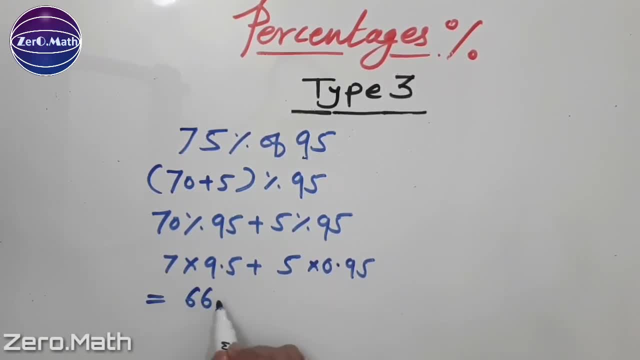 7 into 9.5 is 66.5.. Plus 5 into 0.95 is 4.75.. So our answer is 71.25.. How to perform this multiplication in mind, you can see the previous example. 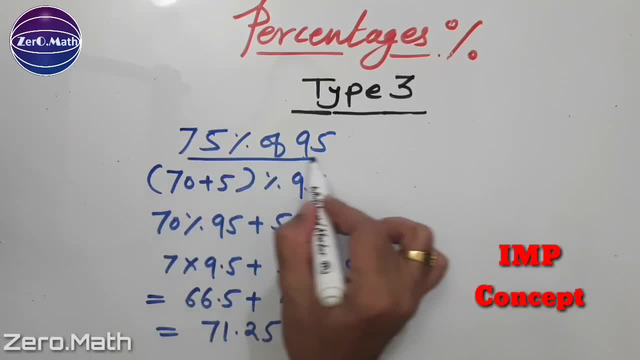 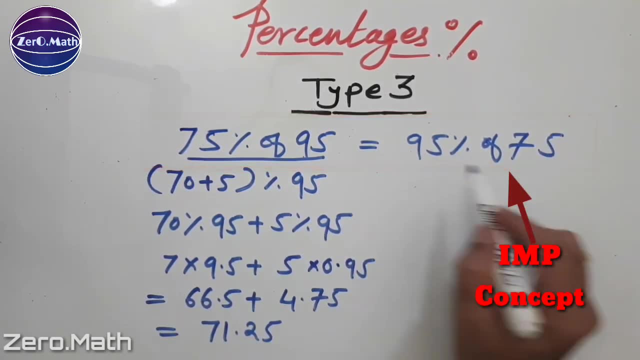 I would like to highlight one important thing here. When we say 75% of 95,, it is equal to 95% of 75. Both means the same thing. Let's see how. So 95% of 75,, let's try to solve it. So 95, I can represent. 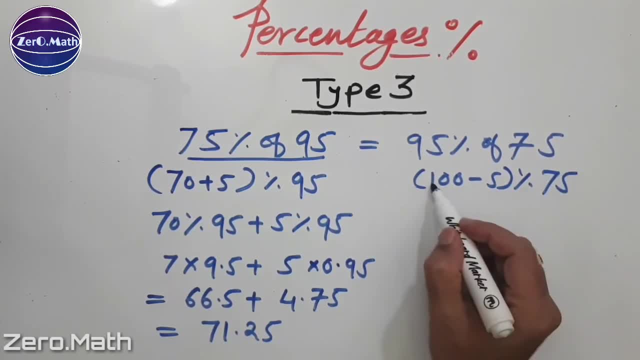 I can split it as 100 minus 5% of 75.. So 100% of 75 minus 5% of 75. So 100% of 75 is 75 minus 5% of 75.. I can write: 5 into 1% of 75 is 0.75.. So my answer is: 75 minus 5 into 0.75 is 3.75, which is equal to 71.25.. 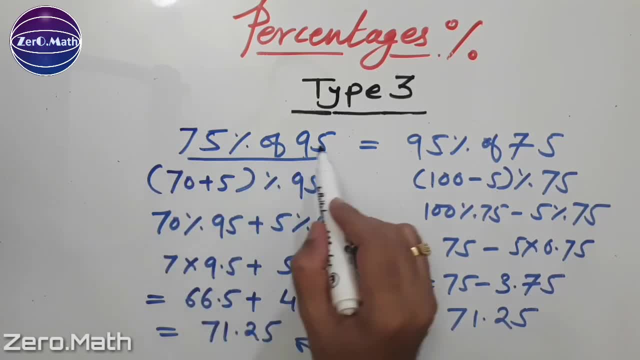 You can see If I calculate 75% of 95 or 95% of 75, both are going to give me the same result. However, the calculation part in 95% of 75 is a bit less because I am splitting it as 100 minus 5.. And always calculation with respect to 100 are a bit easy. That's why I would recommend to do it this way.